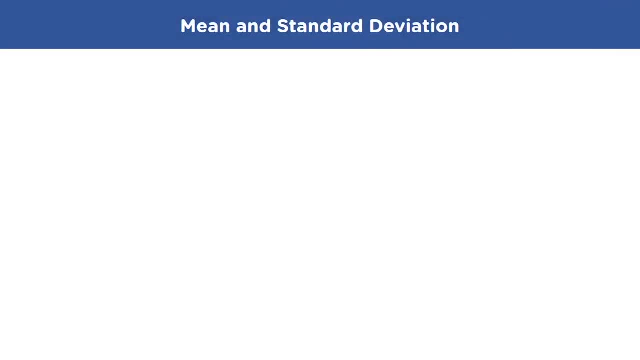 of them. Let's discuss the mean and standard deviation associated with it. Suppose we are sampling from a population with mean mu and a standard deviation sigma. Let x be the random variable representing the sample mean of n independently drawn observations. Then we can say that the mean of the sample is equal to the sample distribution of n independently. 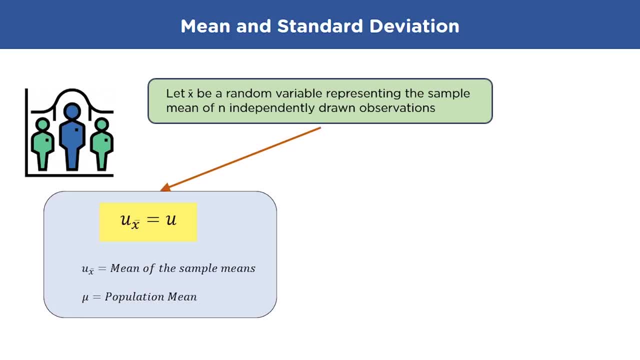 drawn observations, Then we can say that the mean of the sample means is equal to the population mean, which is mu x bar, is equal to mu, where mu x bar represents the mean of the sample means and mu represents the population mean. On other hand, the standard, 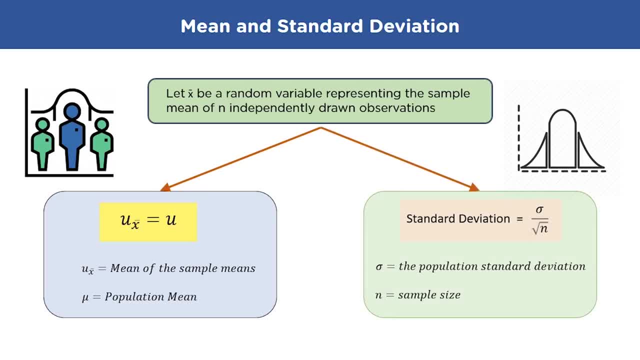 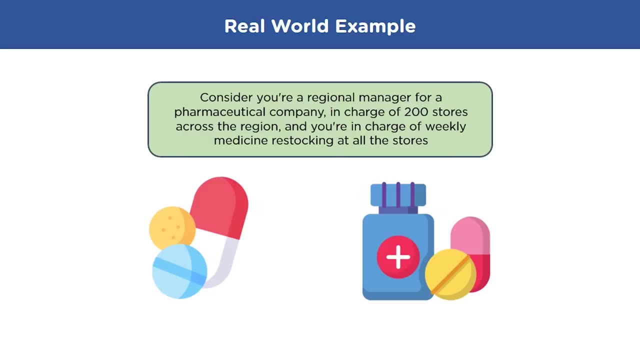 deviation of the sampling distribution will be equal to the population of the total standard deviation upon the under root of sample size. Let's understand this more clearly by taking a real world example. Suppose you are a regional manager pharmaceutical company in charge of 200 stores across the region and you are in charge of weekly medicine restocking at all. 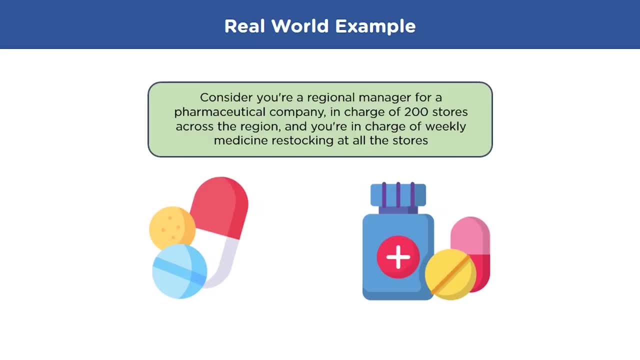 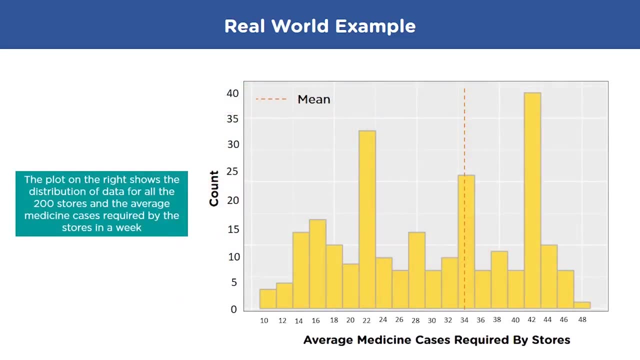 at all of them. You need to know how many cases to order weekly for each store in order to reduce the amount of inventory that expires. The plot on the right hand side shows the distribution of all the 200 stores and average medicine cases required by each of the stores in a week. 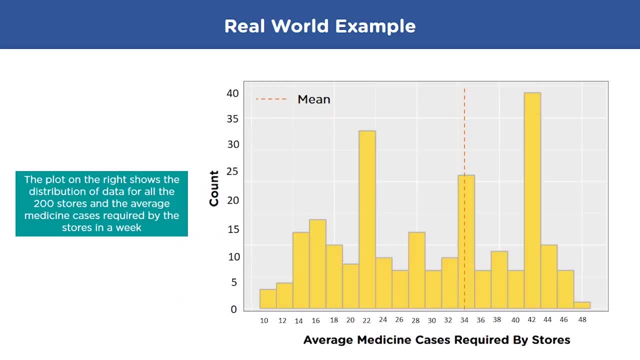 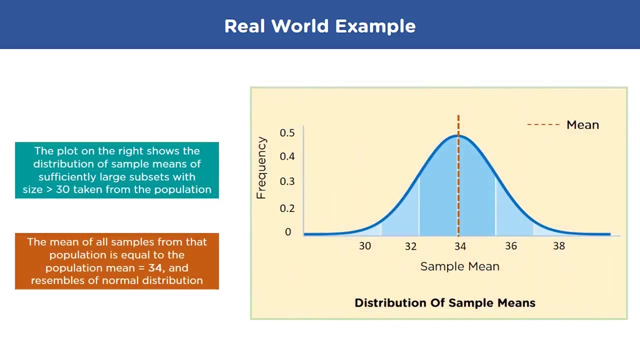 The red line represents the average cases required, which is equal to 34.. You know there has to be a better way to arrive at a reasonable answer that doesn't entail visiting every single store in your area and obtaining their weekly sales figure. You can apply the central limit theorem to this problem now that you understand the concept. 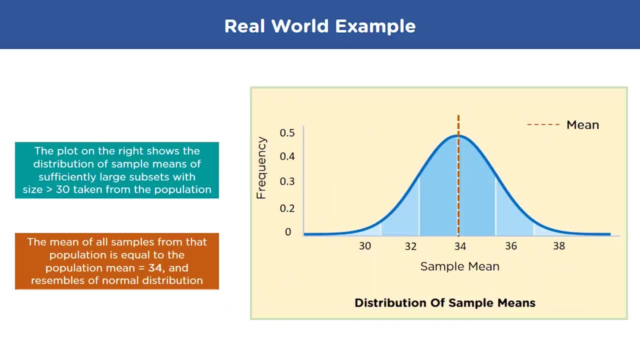 We already knew the central limit theorem, when applied to arrival problems, aids in balancing the time and cost of gathering the data required to draw the conclusions about the data. So here you can see. the plot on the right hand side shows the distribution of sample means of the sufficiently large subsets taken from the population. 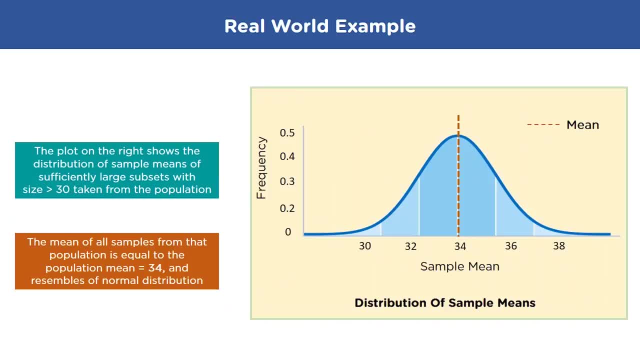 Sample size greater than 30 will be sufficient enough to get the normal bell curve. The mean of all the samples taken from that population mean is equal to 34, which is equal to the sample mean of the population. If you plot the sample means, you will get a normal distribution which is a form for. 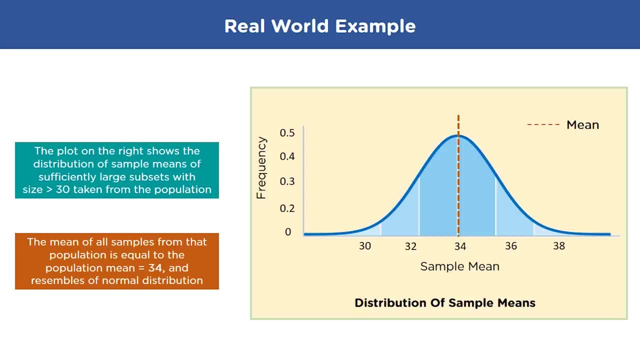 bell curve. If these samples meet the central limit theorem criteria, you can assume the distribution of the sample means can be approximated to the normal distribution. Now you know how to apply the central limit theorem in a real world problem. Let's discuss some assumptions behind the central limit theorem. 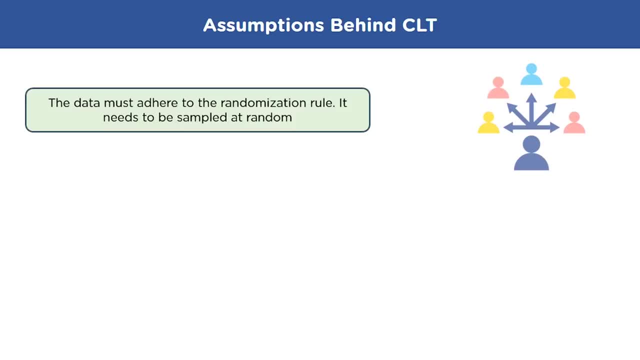 The first one is the randomization condition. The data must be sampled at randomly and it must adhere to the randomization rule. The second one is the independence assumption. The sample value must be independent of each other. This means that the occurrence of one event has no influence on the next event. 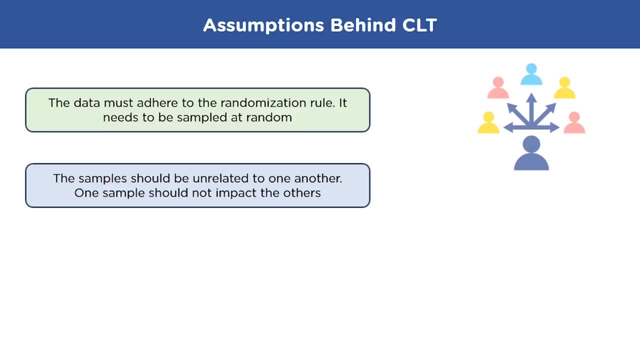 Usually, if we know that people or items were selected randomly, we can assume that the independence assumption is met. The third and the last one is the 10% condition. This states that when the sample is drawn without replacement, the sample size, which is n, should be no more than the 10% of the population. 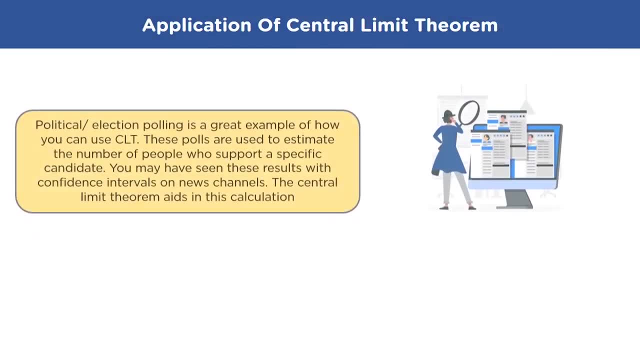 Let's now discuss some application of the central limit theorem. Political and election polling is a great example to show how you can use the central limit theorem. These post results are used to estimate the number of people who support a specific population. These post results are used to estimate the number of people who support a specific population. 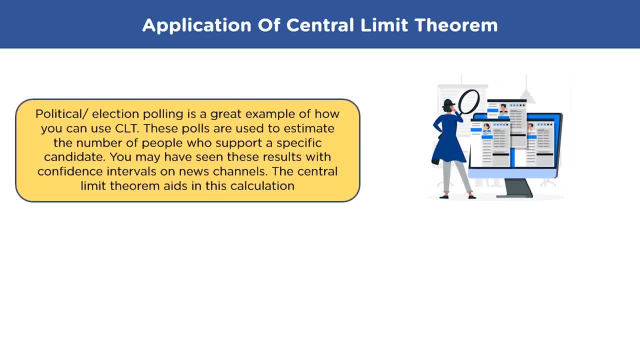 Let's now discuss some application of the central limit theorem. These post results are used to estimate the number of people who support a specific candidate, To calculate the confidence interval which is shown on the news channel. the central limit theorem is very useful in this. 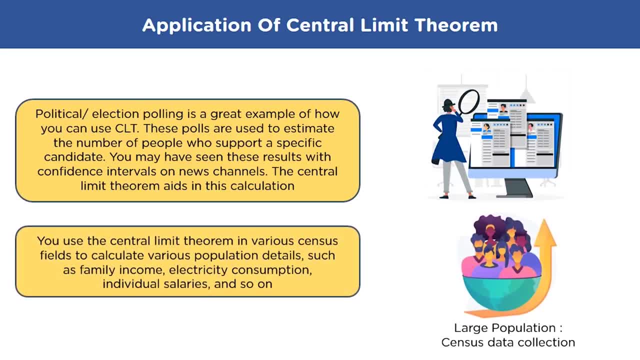 One more place where you can use the central limit theorem is the census data. You use the central limit theorem to calculate the various population details, such as family income, electricity consumption, individual salaries and so on. Now that we have a good understanding of the central limit theorem, its theories and application, 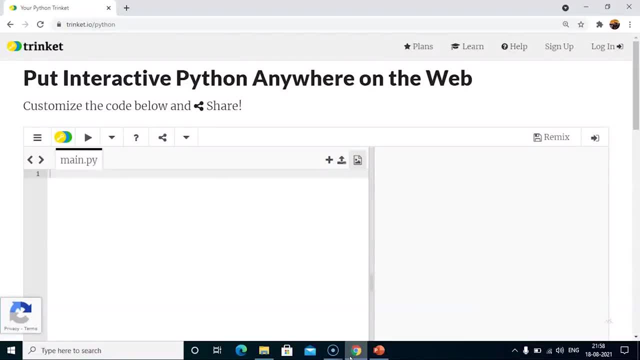 let's see a demo in python to understand it more clearly. Here we are on an online compiler. We will discuss the CLT by taking a dice example. A dice is a different number on each side, ranging from 1 to 6.. 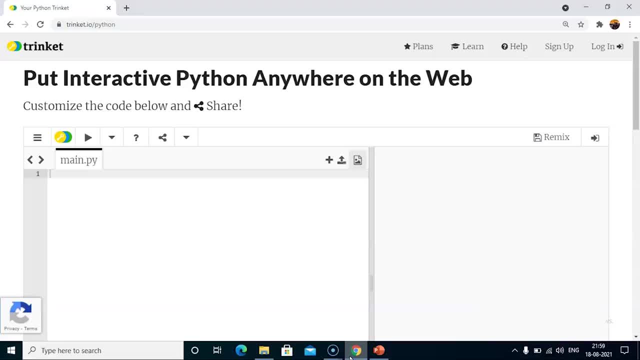 Each number has a 1 in 6 chances of appearing on a roll. Given all the equal likelihood, the dispersion of the numbers that come up from a dice roll is uniform. Let's start by importing some necessary libraries. We'll import the numpy first. 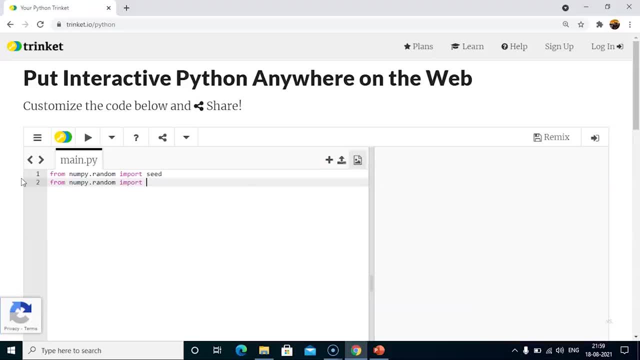 From numpyrandom we'll import the random function, which will be used to generate the random integers. We'll also import the mean function from the numpy. We'll set the seed. Now we'll write the function to generate the random numbers. The randit function will generate a number ranging from 1 to 6.. 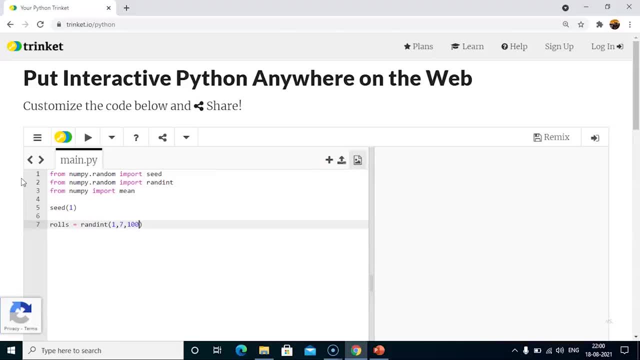 We have taken the 100 because the example will generate the print samples of 100 dice rolls along with the mean. Print the rolls and then we'll print the mean of the rolls. So when we run this code we'll get the following result: 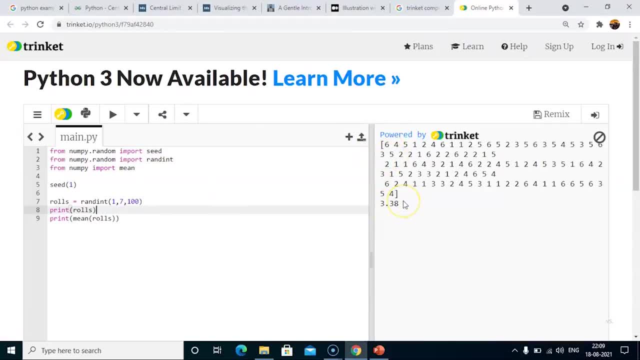 You see, we have the 100 numbers and the mean of this number is 3.38.. Now we'll repeat the process 1000 times. This will give you the result of 1000 sample means. According to the CLT, the result of the sample means will be Gaussian. 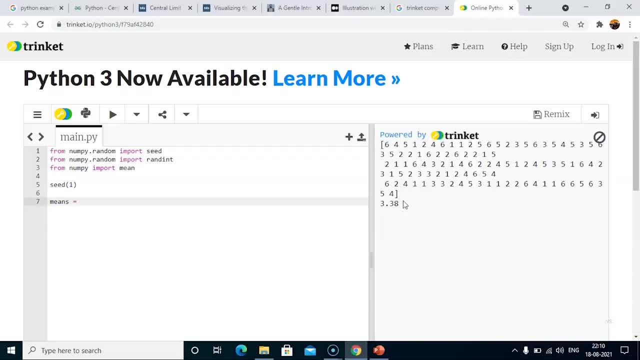 So we'll change this code from here. Means will be equal to mean of this random integers. We'll take from 1,7,100 and this will be 4 in range of 1000.. Now we'll plot this distribution. We'll use the piplot function. 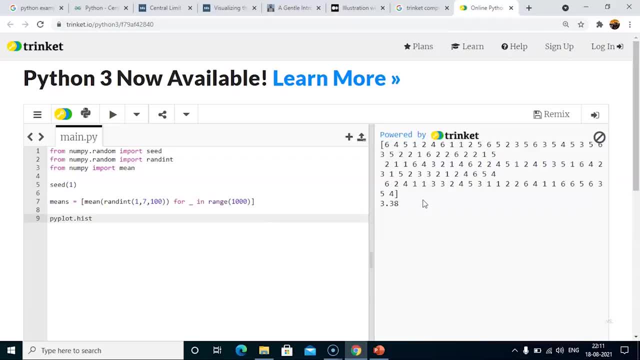 We'll get the graph as a histogram graph, So we'll plot it in that. Means and piplot. Now we'll plot this distribution. We'll use the piplot function. We'll get the graph as a histogram graph, So we'll plot it in that. 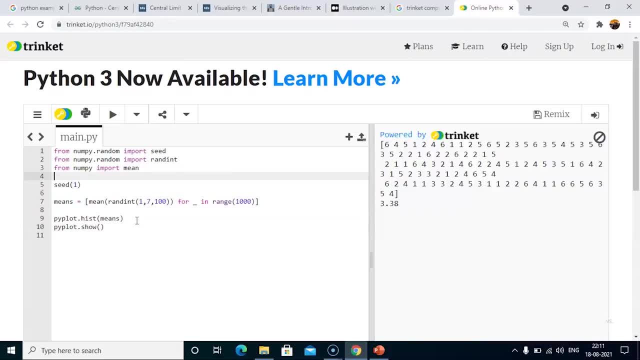 Means and piplotshow. Let's recheck our code. We have the random integers function. We have the feed. Okay, we have imported the mean. We have not imported the matplot library. So from matplot library we'll import piplot. 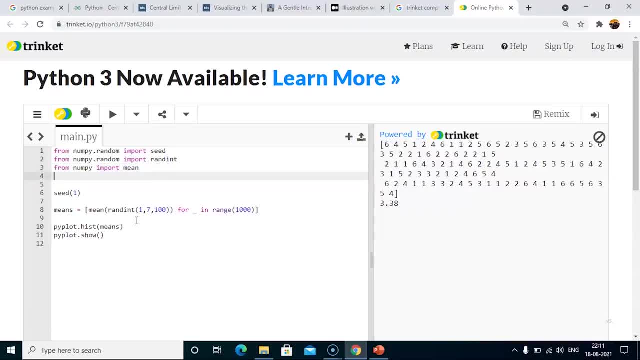 Now I think everything is in place and let's try to run this code. Yep, you can see this graph is a histogram graph in a shape of a bell curve And if you see closely, the mean is 4 in range of 1000.. 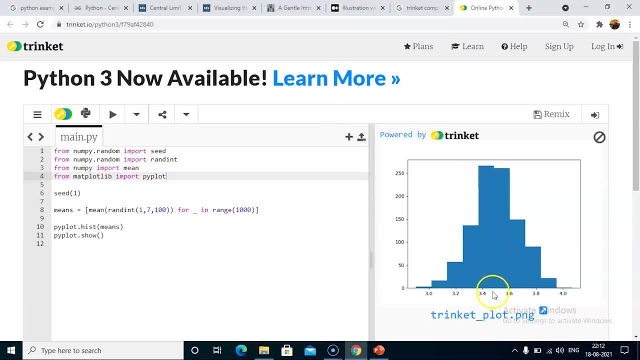 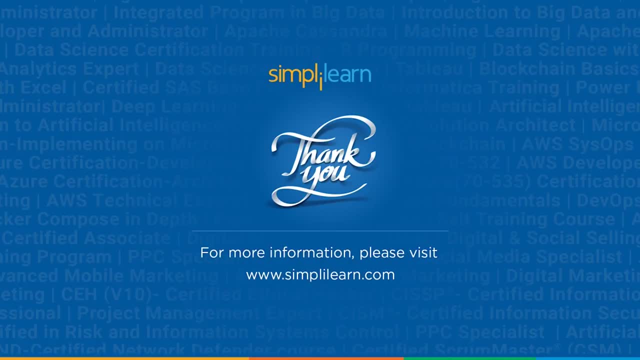 closely. the mean is closely to 3.4.. So that's it for this tutorial. Thank you for being here and watch out for more videos from us. If you have any doubts and queries regarding the central limit theorem, you can post it. 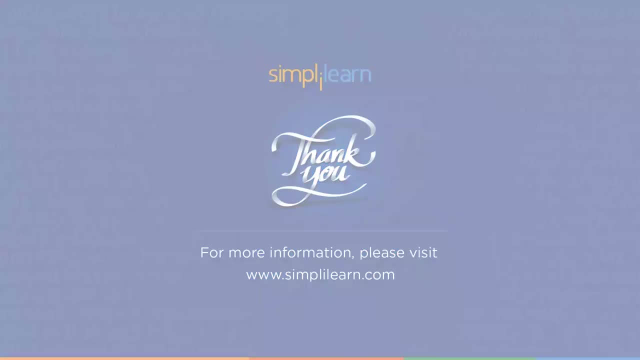 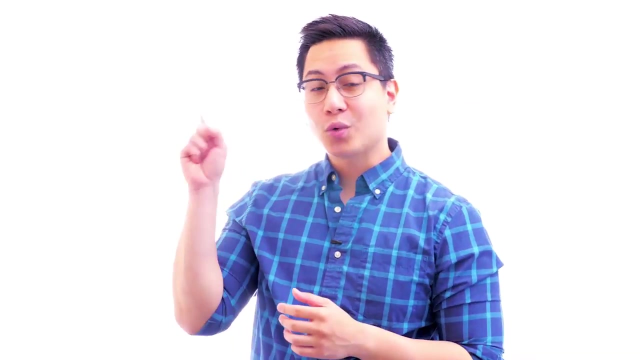 in the comment section. Until then, keep learning and stay tuned to Simply Learn Hi there. if you liked this video, subscribe to the Simply Learn YouTube channel and click here to watch similar videos. To nerd up and get certified: click here. 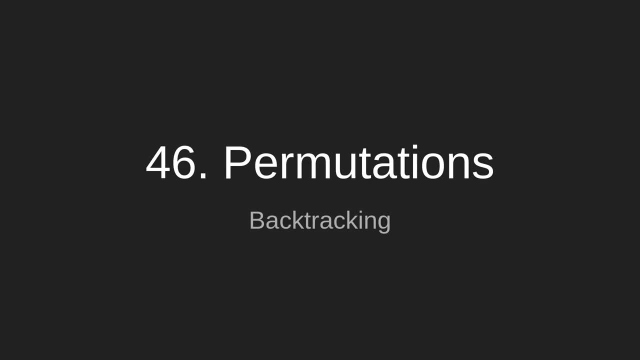 Hey, how's it going? This is Computer Bread and in this video we are going to look at the litcode problem, number 46, called permutations. This problem will serve as an introduction to backtracking, So the description of this problem is quite simple. So, given a collection of distinct 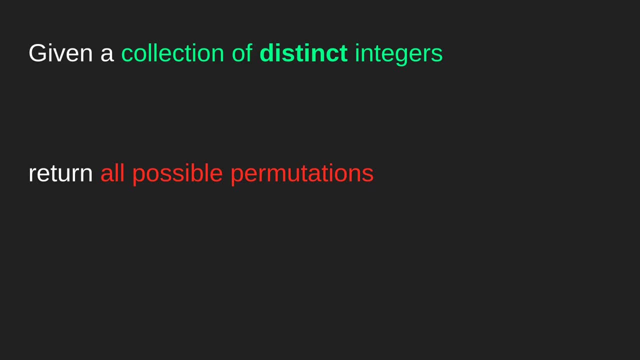 integers return all possible permutations. So we are given an array we call nums, that will contain numbers like 1, 2 and 3 and we want to output all the possible permutations like 1, 2, 3,, 1, 3, 2,.